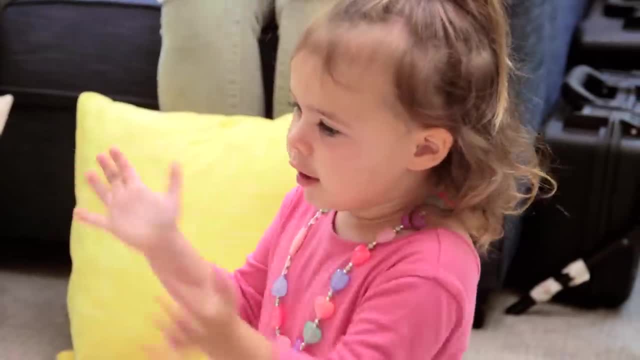 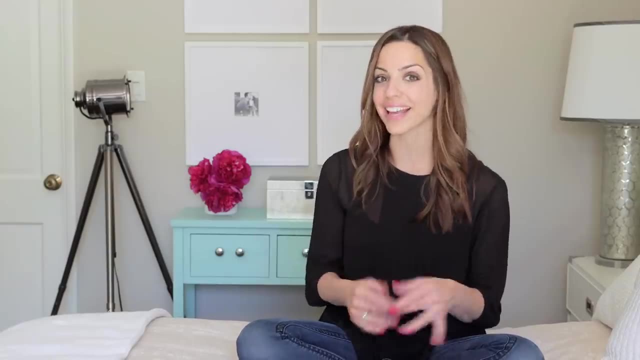 Hey guys, So my kids love magic and with their cousin visiting, they wanted to put on their own show. So we had to find tricks that don't require too much sleight of hand and then, with my help, prepping, they could actually perform by themselves. 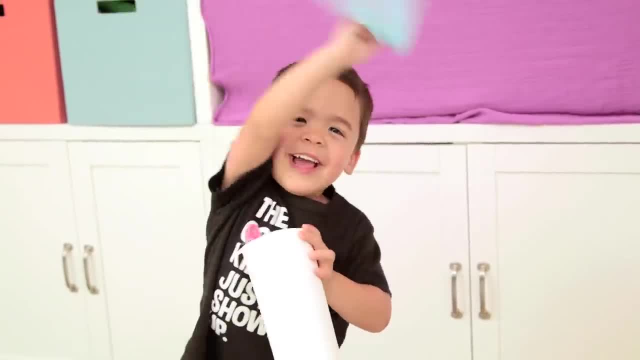 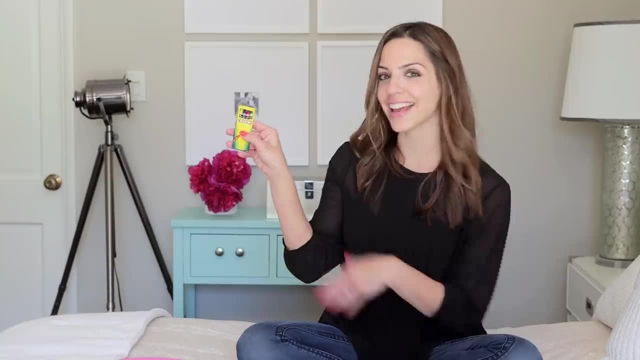 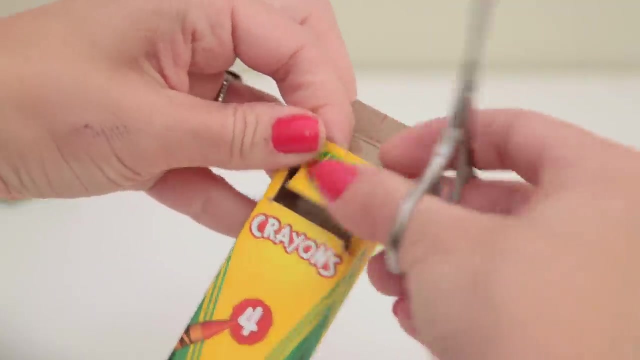 So, without further ado, our five favorite magic tricks for kids. Welcome to the Magic Show. So number one: disappearing crayons. Now you see them, now you don't. So these are just like a pack of crayons you get at a restaurant. I cut out a window, tape the crayons together and then the key is you chop them in half. 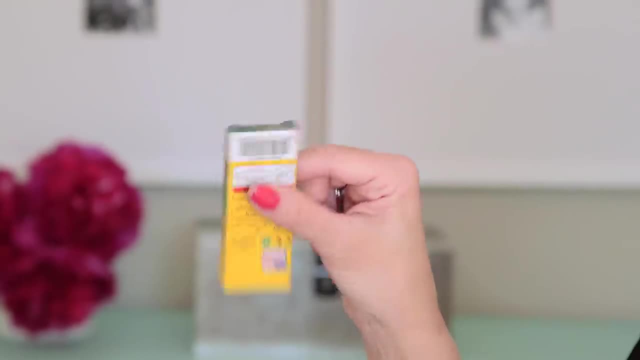 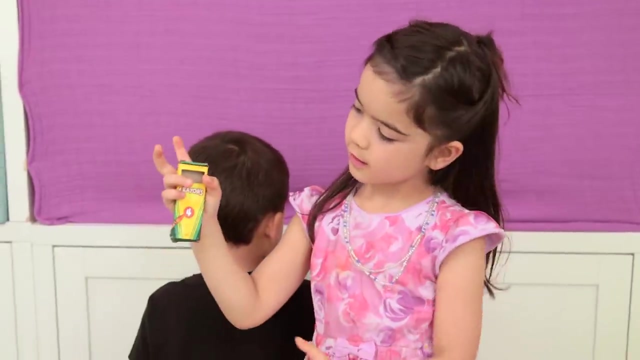 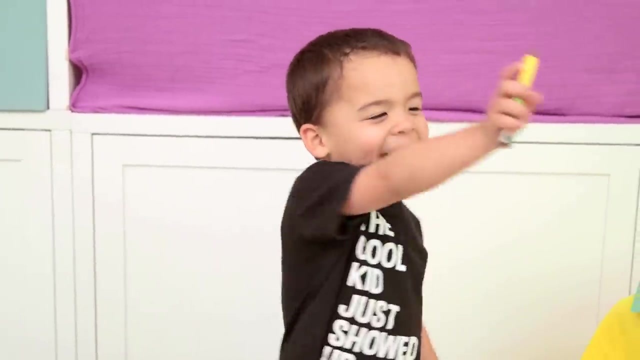 So when you apply pressure, they're up. Let that go. they fall down. Bring them back by flipping over the box. The kids love doing this. one, Boss, we have disappearing crayons. Where'd they go? Whoa. Or you could just throw them out of the box And then whoa. 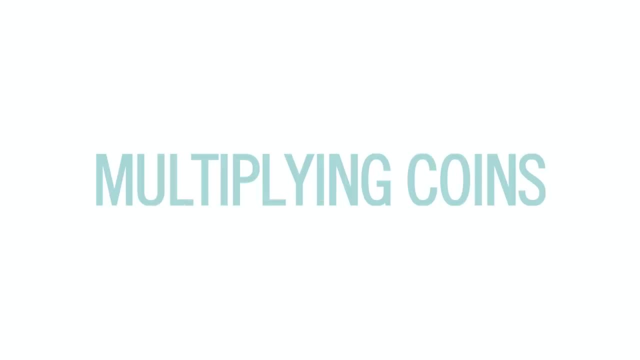 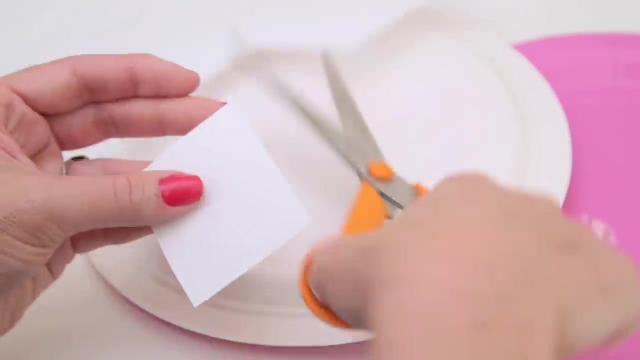 This is a bear Next up. multiplying coins, You guys ready. One, two, three. And to do this, you guys see the back of the paper plate. We've just taped on a little piece of paper to create a pocket. tuck our quarters in and voila, Presley nailed this. 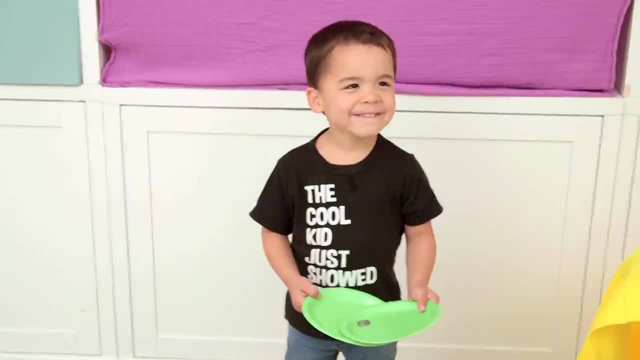 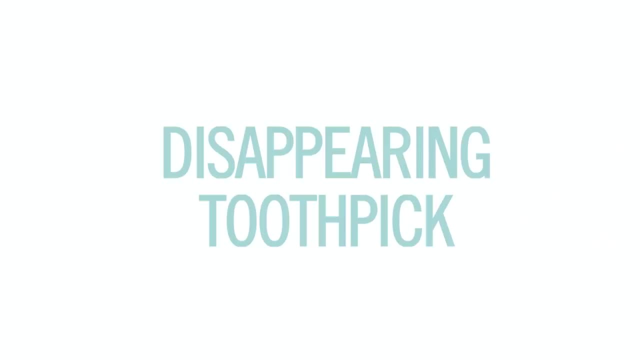 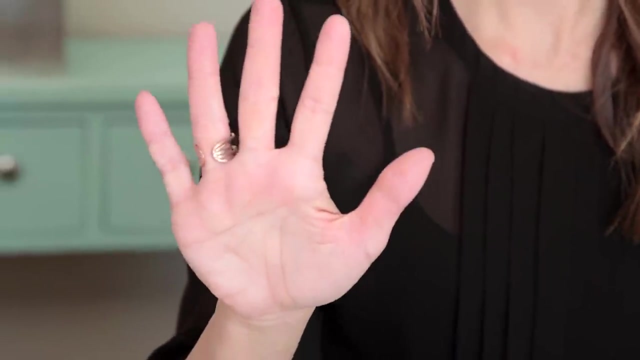 Oh, Ford showed a little too much pocket. What The test. totally bought it. Number three: the disappearing toothpick. Where'd it go? Oh, there it is. Oh no, I gotta work on my magician acting. Leave that to the kids. 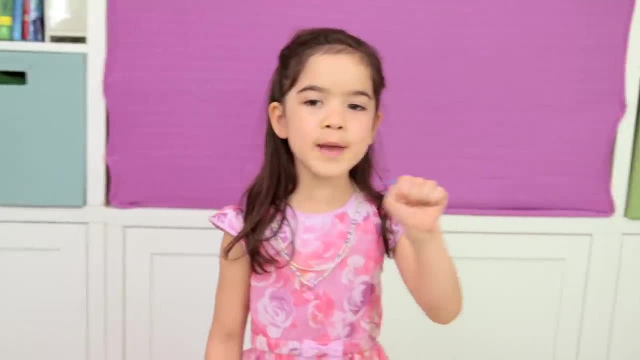 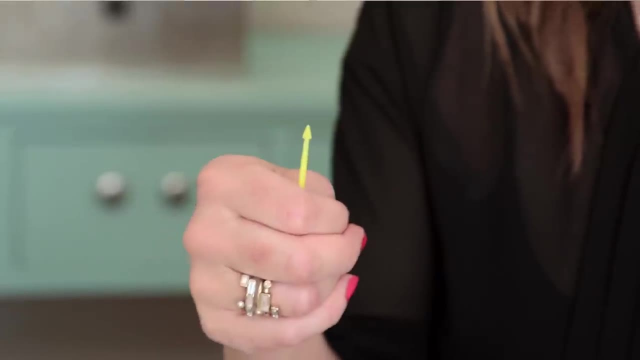 Everybody. you see this. Yes, I'm gonna make it disappear. What, What? All you need to do is tape this toothpick onto your thumb and it's such a fun and easy magic trick for kids to get right away. Whoa. 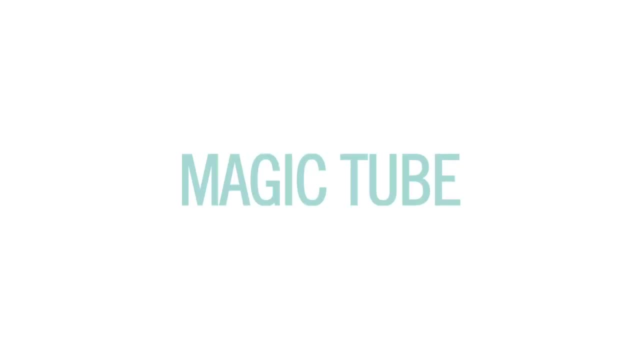 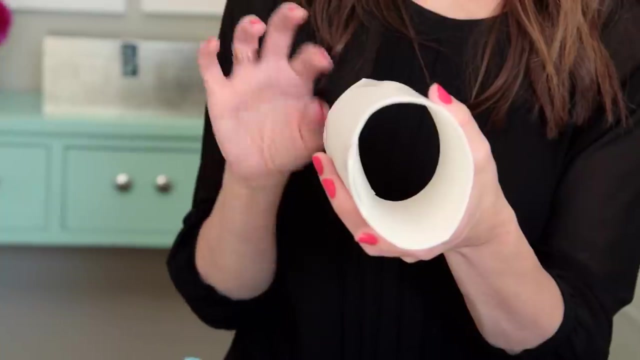 Oh, Next up, we've got our magic tube. Now this looks just like a normal, ordinary tube, until you- Oh, Where'd that come from? I was looking for this. All right, you guys. so this is actually an optical illusion. 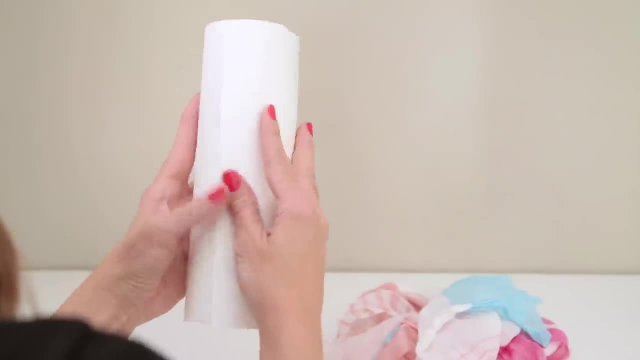 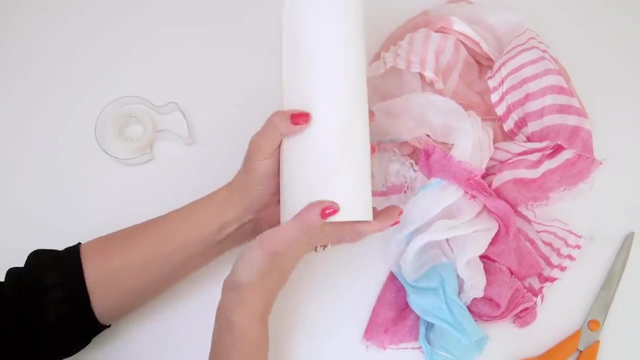 It's two tubes and how we made this. you roll up a piece of cardstock, then you roll a second piece up, the same on one end but more of a cone shape on the other. Put them together, tuck in your tissue.